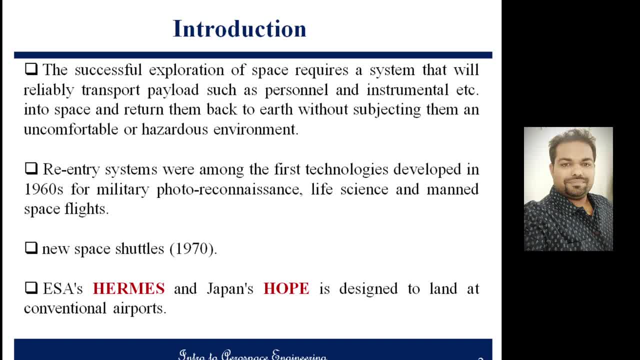 the earth, followed by the safe landing. So you might have seen several examples in the Hollywood movies. So these are some of the examples in real-time scenario where re-entry into the earth atmosphere have been accomplished. And also you might have seen that famous example right in 2003,. 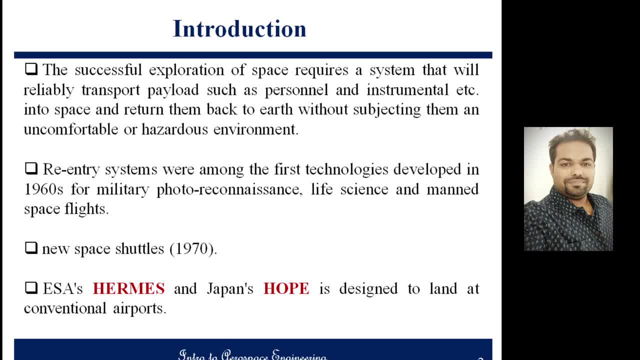 right on Kalpana Chawla incident, right when that space shuttle was entering into the earth atmosphere and it was exploded because of the phenomena called re-entry heating. It was not able to sustain that heat and it has broke into the two parts. One part went. 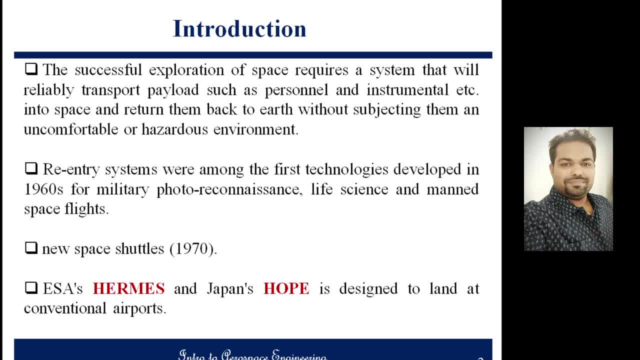 into the space. another part came on the earth. That phenomena may have been, but after that incident, right, lot of researchers have come up with significant, you know, solutions to avoid the aerodynamic heating. Still, aerodynamic heating or re-entry heating, is a subject of. 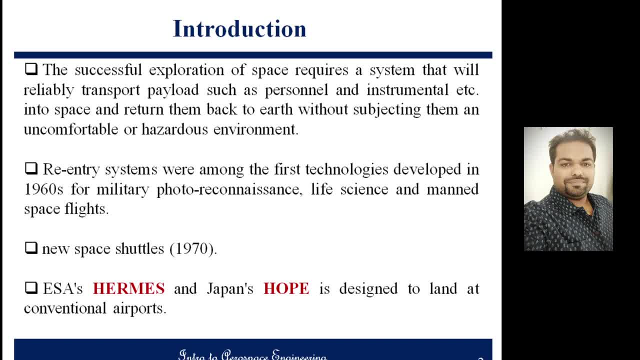 research, Lot of research is going on. So in order to you know, understand this aerodynamic heating, the researches must have in-depth understanding of high-speed aerodyamics. So lot of lot of parametric studies need to be done before come before come to the conclusion of fully optimised design for space. 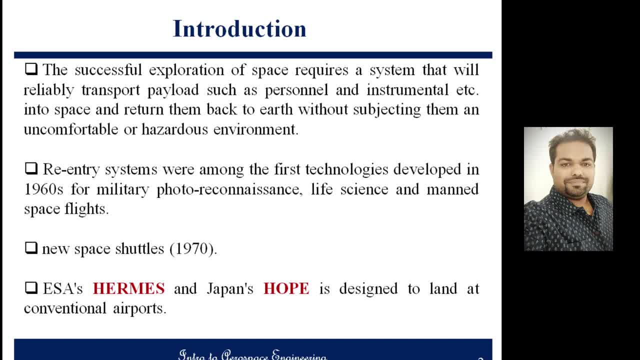 exploration. So if you look at, look at uh statement, description, statement of a space experiment, a facility's answering cases, can you see how it might be suitable for throughout the world. So anyway, in reality it's tricky, but there's a vast, there's a lot of information. 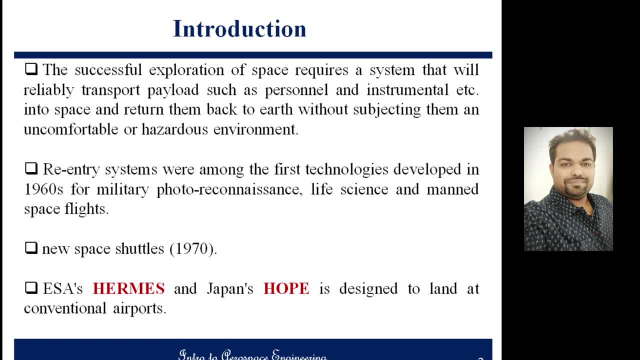 the history of, you know, space exploration. space exploration just started uh immediately after the world war ii in 1960s. you know uh, russia started the space race and after that it is still continuing, still continuing and the coming future, uh, warfare and all you know necessary things will. 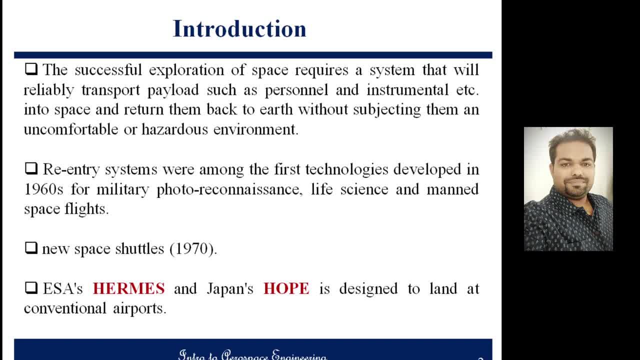 be, uh, you know, uh, dominated by the space shuttles right and and, and and. to accomplish that and to understand the space, you need a spacecraft. so re-entry systems were among the first technologies developed in 1960s for military photo reconnaissance, life science and manned space. 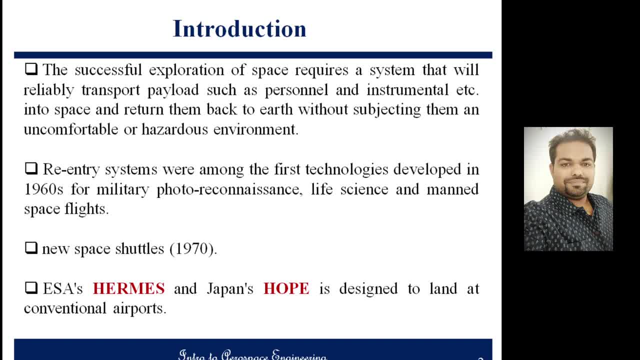 flights by 1970s. it led to the development of new space atoms. today, today we look at today, space technology has developed to space planes which intend to go and come back regularly from earth to space station. if we look at the example, particularly european space agency harness and japan's hope, these 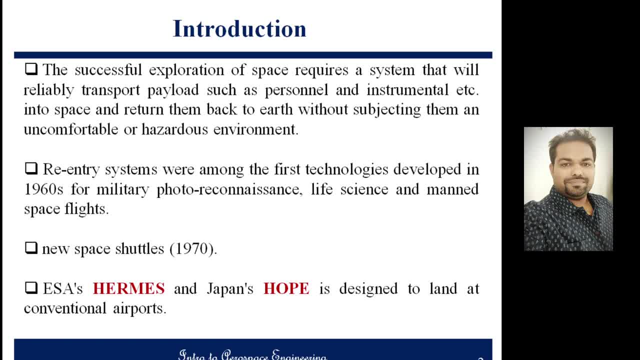 spacecraft are designed to lend like an conventional aircraft on the airport. as i said, that spacecraft, if we look at the configuration of a spacecraft, it will be similar, like an aircraft, and it has to be launched with the help of a launching vehicle. a launching vehicle will be a rocket with the help. 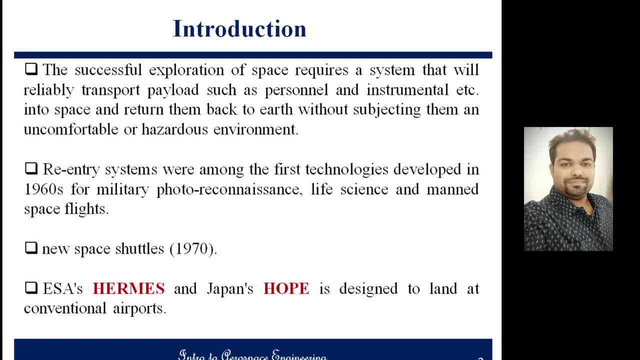 of that. we used to send the spacecraft into the outer space. when it is going to be land, it will be landing with help of its own engine, so it is fitted with the engine. so when it is going to be land on the, on the earth's surface, it will be landing like that, like an aircraft after. 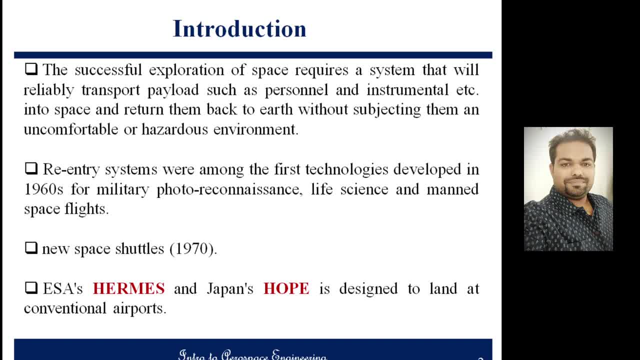 after crossing all those aerodynamic heating stages and finally land on the earth. so, as i mentioned that you know, esa, helms right and and japan's hope. these are, uh, particularly two famous spacecraft which which were particularly designed to land on the airport like an aircraft. so if you look at the helms, helms was basically a joint venture. it was not a single country. 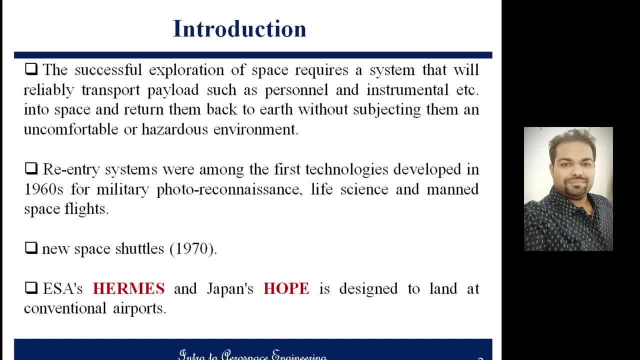 which was working on the helms project. so helms spacecraft is the result of decades-long collaboration between nasa, european space agency, ROSCOM, russian and japan aerospace exploration agency and ISRO- ISRO, our indian. so they are planning, uh, basically, to develop it basically soon right for space exploration, particularly from earth to mars orbit and return back. 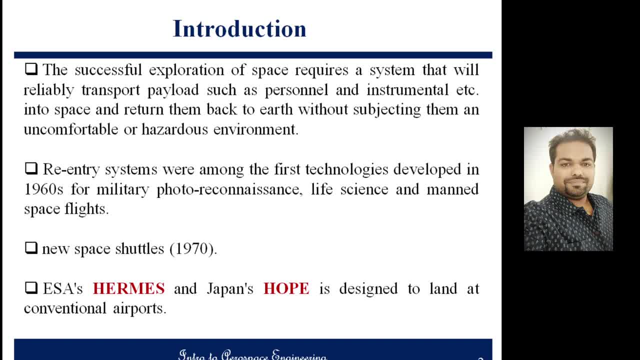 so first, you know, helms project was started by the french center national company in 1975. later it was taken by the european space agency. so it was basically being designed taking into consider that space travel should be very easy and convenient. at any time you can go to the space, explore, return back, so in 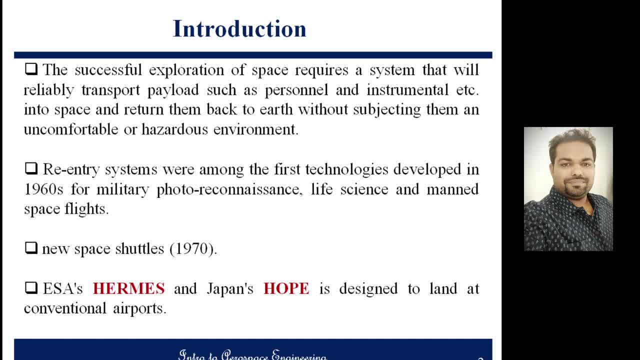 coming future, it will you know, come into the effect. so these collaborative work is going to be end by 2029. so we are, we are expecting that by 2029 we will be ready with the future space craft. Next one is japan hopes particularly hope was Japanese experimental space plane project. 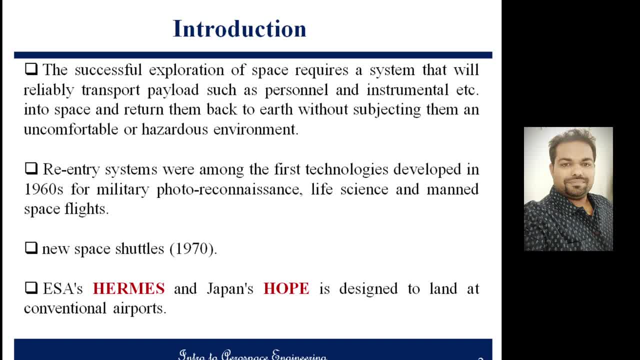 designed by partnership between national aerospace space development agency and national aerospace laboratory of japan. now it is known as basically JAXA. JAXA is japan aerospace exploration agency, so these two agencies basically combinedly known as now JAXA. so it was positions for most of its lifetime as one of the main japanese contribution to 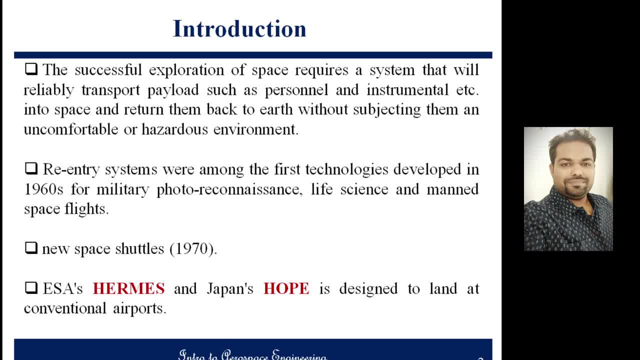 the international space station, another being japanese experimental module. the project was eventually cancelled in 2003, by which point test flights of subscale tested had been successfully conducted. so they have conducted the you know flight test and as well as real-time test. but it has been such down into down three and after that no more work has been done but this. 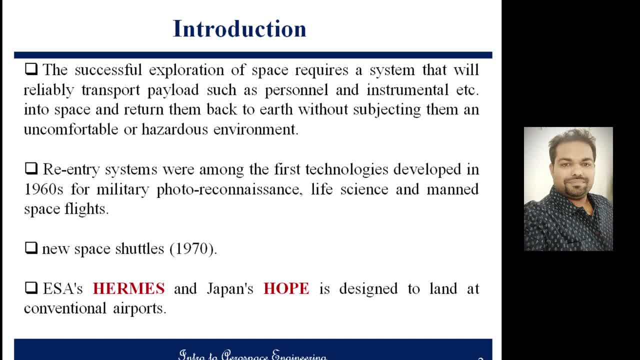 were designed particularly to land on the conventional airports. from any airports right, they can land. so return back to the topic again, as i said that for accomplishing a successful exploration to space we need a spacecraft now. spacecraft need to be designed in such a way that it should encounter all the forces which will come in this way, like aerodynamic heating, re-entry heat. 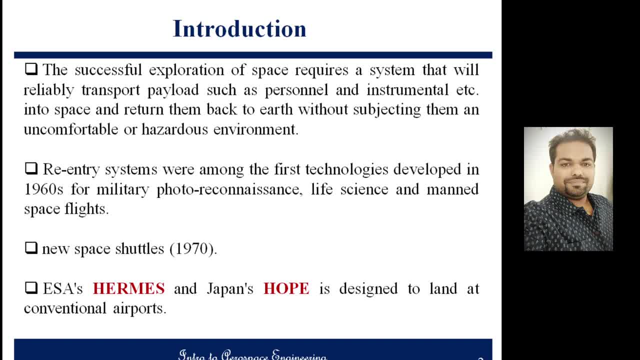 heating and atmospheric turbulence as well. so for entering into the atmospheric and non-atmospheric planet, the problem involves is reducing the spacecraft speed. how to reduce the speed? because in the outer space there is no resistance. when there is no resistance, the motion which have been provided to it will be the main, almost same. it is very difficult to reduce the speed. 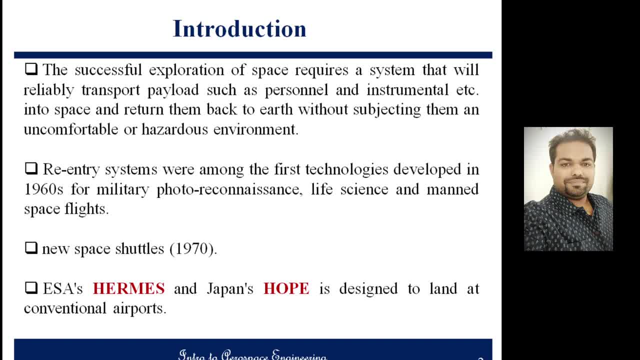 how to do that. that is a big question in front of a scientist and researcher, so they are looking for the solution for it. another big problem is aerodynamic heating. how to minimize that? we cannot completely avoid it, but you can minimize it. for that lot of you know, work has been done. we are having thermal shield system. 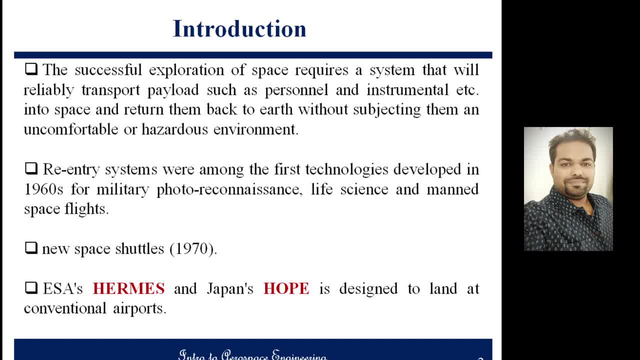 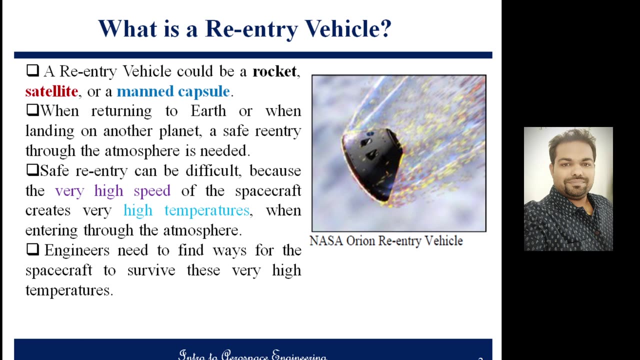 or we can use thermal barrier coating, special coating at the nose, to avoid the re-entry heating, but still some more modifications are possible that need to be done. so so if you look at what is basically re-entry vehicle, if somebody asks you what is re-entry vehicle, a re-entry vehicle could be a rocket, could be a satellite or can be a manned capsule. 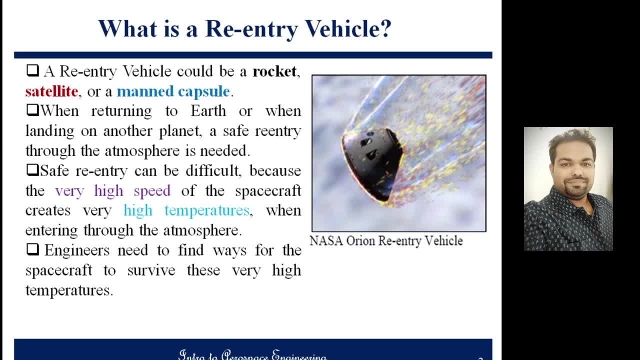 so when returning to the earth or when landing on the another planet, a safe re-entry to the atmosphere is needed. so safe re-entry can be difficult because very because of the very, very high speed of this spacecraft. so we need to be careful about that spacecraft, which creates very high temperature when entering through the earth atmosphere. 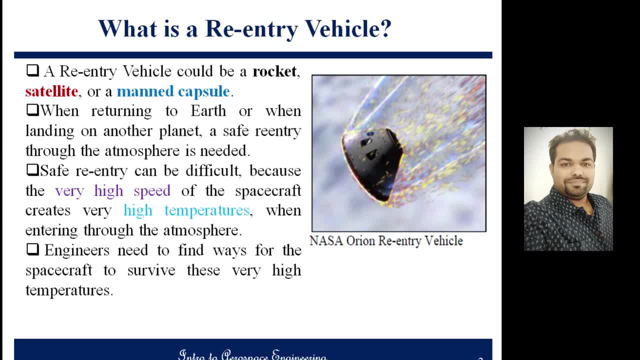 so engineers need to be find ways for the spacecraft to survive these very high temperature environments. so this is the famous example of the manned capsule nasa orion re-entry vehicle. so in front of researchers, these are the big problems: how to survive the re-entry heating- and for that lot of modifications has been done. it's a lot of research is going on. 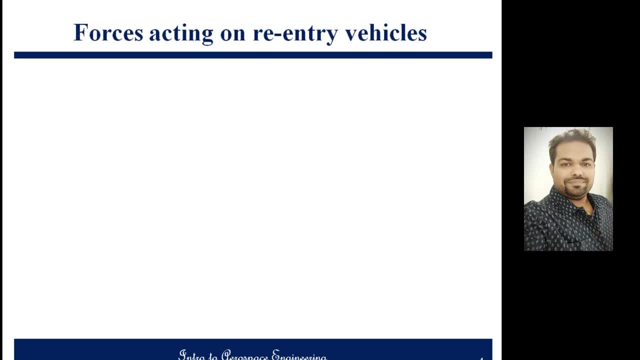 so forces acting on re-entry vehicle. ap categorize the forces which will come on the way of a re-entry vehicle. they can be classified into three major forces. one is gravitational force acting towards the center of planet from where it is getting entered into the earth atmosphere. 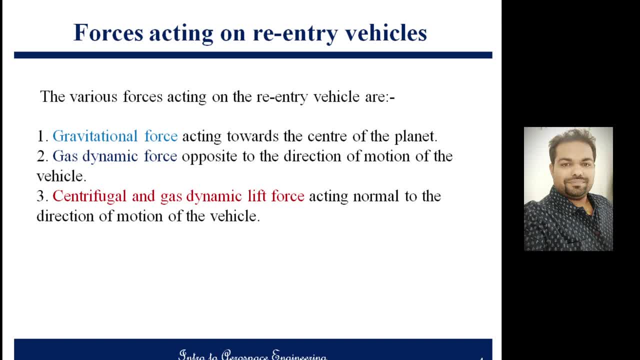 so now question will arise: whether, in you know space, gravitational force is there in space, then some zone, there is some value of gravitational force, right, gravitational force maybe 1 by 6,, 1 by 9.. So that gravitational force will pulling the spacecraft back to the planet, right that? 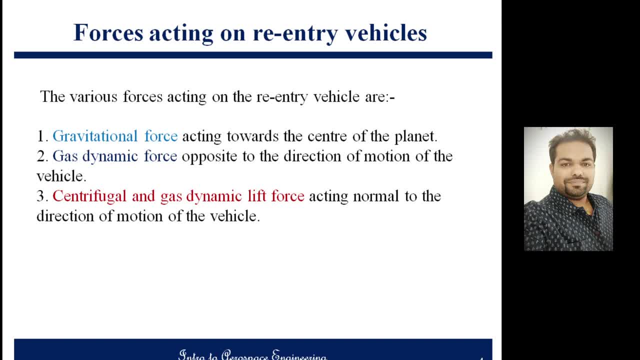 need to be, you know, counter and counter. So gravitational force acting towards the center of planet. Next one is gas dynamic force. opposite to the direction of motion of vehicle and gas dynamic forces will come because of the presence of shock waves right at the surface of the. 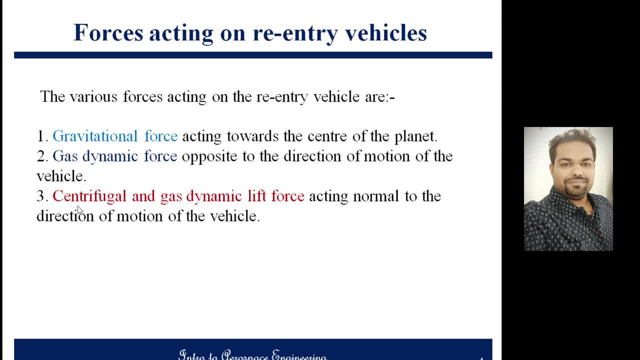 spacecraft. Third force, centrifugal and gas dynamic lift force acting normal to the direction of motion of vehicle that will also try to change the flight path of the re-entry vehicles. So these are the major three forces which would be acting on the surface of re-entry vehicles and 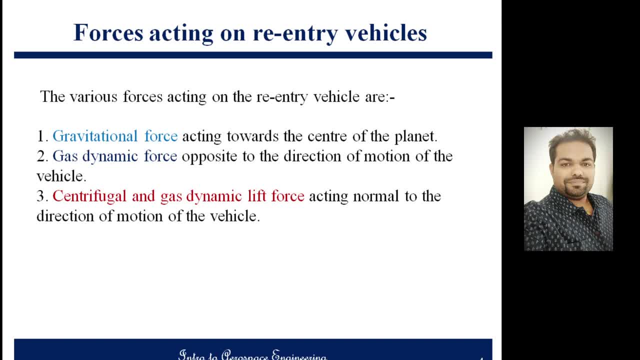 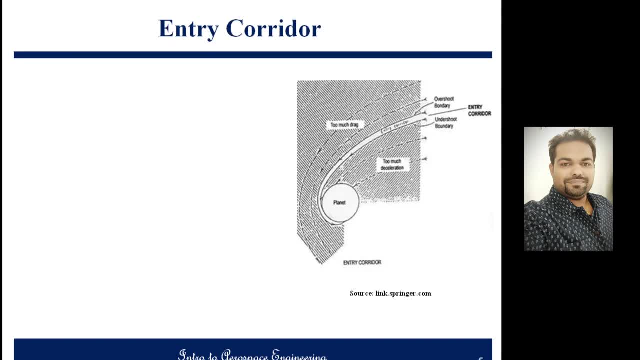 need to be encountered And for encountering these forces you need sufficient power, right powerful engine to counter these forces. If we talk about the entry corridor, there is only particular, you know- passage through which only re-entry is possible. You cannot do re-entry in any way of going from in space. 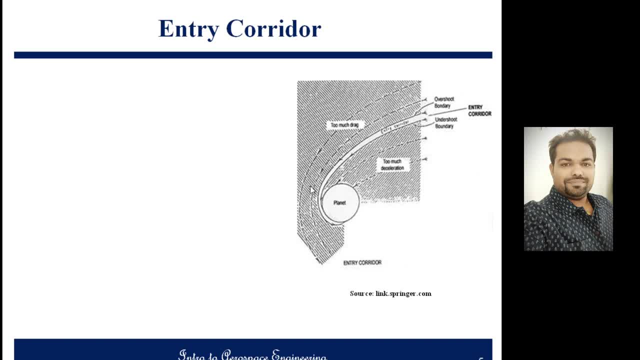 to the earth. So there is only a particular thin zone through which only re-entry is possible. successful re-entry is possible. Otherwise what will happen If you are going this side? there will be too much drag If your space vehicle is going to counter too much. 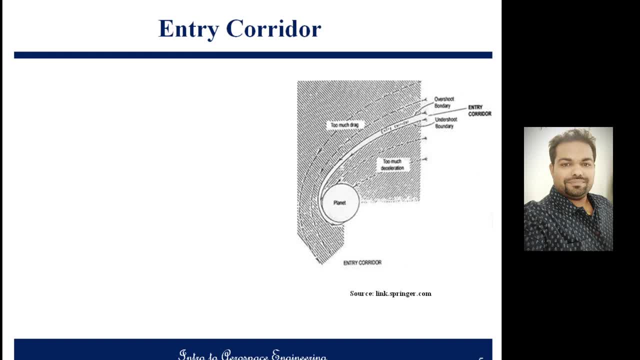 drag and if your space vehicle is going to counter too much drag, you are not able to counter the original Vulcan trading anymore. and due to drag, what will happen? lot of heating of the surface may happen and and and if it is too very, very high track, chances of damage to the uh vehicle is also possible and which will lead to 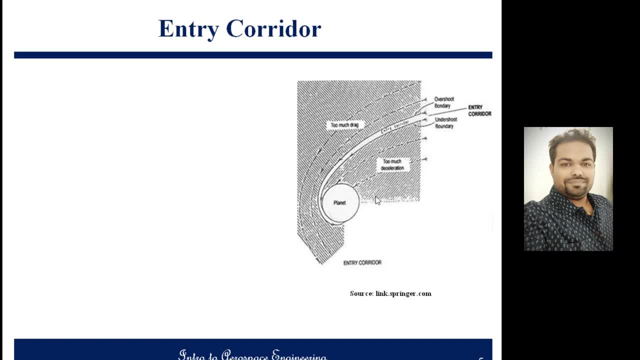 the accident. right, if you are going away from this. uh, you know, corridor, here, deceleration will be too much, too much low. you may not be able to cross the magnetic field of the earth atmosphere, all right. so there is only particular thin zone right through which only successful re-entry is. 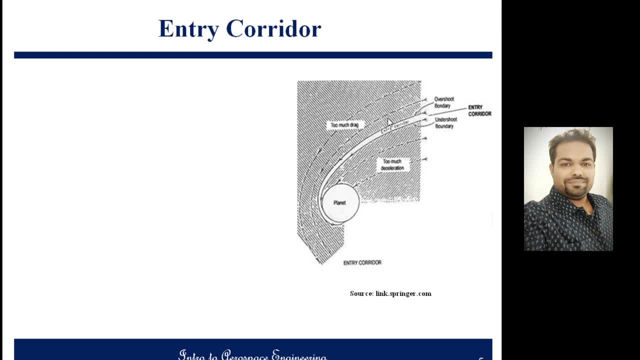 possible. so outer zone. if you look at the boundaries of these, one is called overshoot boundary and is called undershoot boundary. so these are the maximum minimum condition right up to which you can re-enter into the earth atmosphere or you can do the entry into the 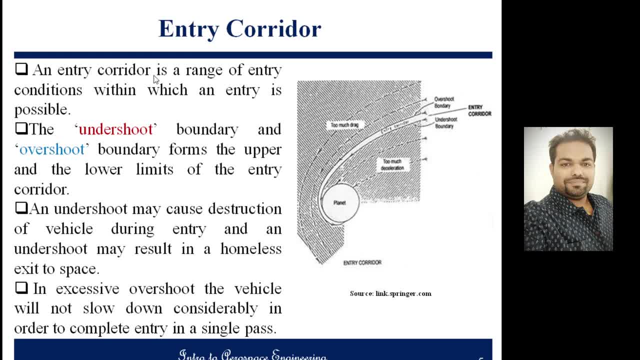 planet. so an entry corridor is a range of entry conditions within which an entry is possible. undershoot boundary and overshoot boundary forms the upper and lower limits of the entry corridor, as clearly mentioned here. so so this is the big problem, uh, uh, basically, uh, so you have to go through only, uh, these uh, very narrow zone, so terrestrial flights. 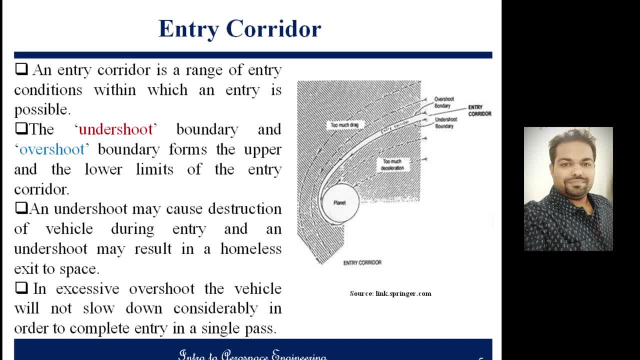 are tolerant of guidance error accompanied by landing approach. there may be some guidance error, so an undershoot may cause destruction of vehicle during entry and an undershoot may result in harmless exit to this space. so if you are going this side right, then it is very difficult, very, very difficult right now, understood, if you are going this side. 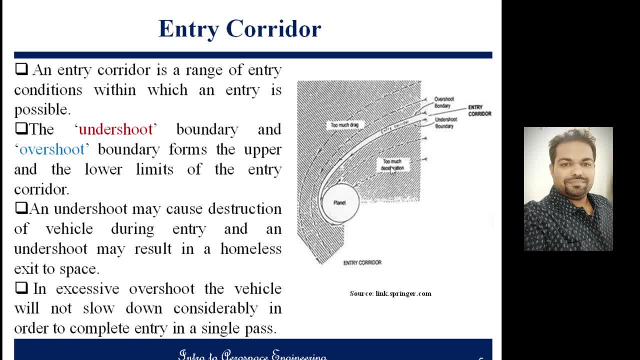 it is very, very difficult to enter into the atmosphere. so you will be still in a space and if you are too much away from it, right, this may cause the structural damage to the vehicle during re-entry. so if the guidance error results in excessive undershoot, right like this, these are the undershoot, these are the excessive condition you look at. 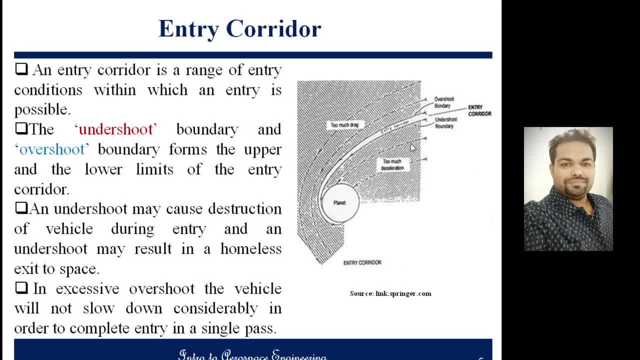 this and this. these are the too much excessive condition. if, due to guidance error, if excessive undershoot happens, the vehicle will enter into atmosphere at an excessively steep angle, thereby experiencing too much deceleration, if the guidance error results in excessive overshoot. similarly, if you are going this side, 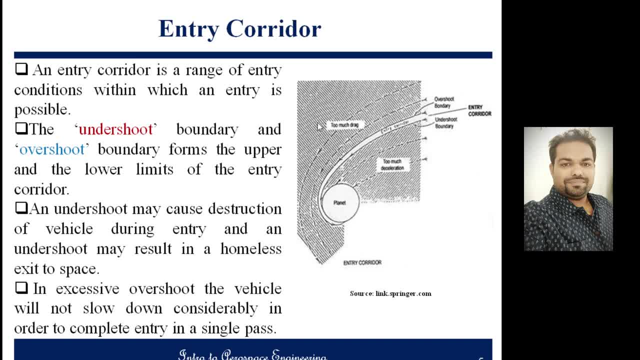 also because of the guidance error. if you are going to the excessive overshoot, in that case vehicle will not slow down considerably in order to complete entry in a single pass, so speed cannot be reduced. that is also very, very difficult right, particularly uh, to complete re-entry. 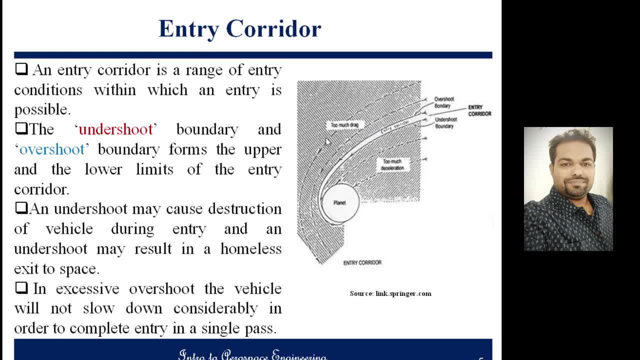 in a single pass it has to be reduced. so in both the condition right either excessive undershoot and excessive overshoot are not recommended. hence the shaded portion represents excessively. overshoot and undershoot are excluded, so there is only particular thin zone which is showing here, through which a successful 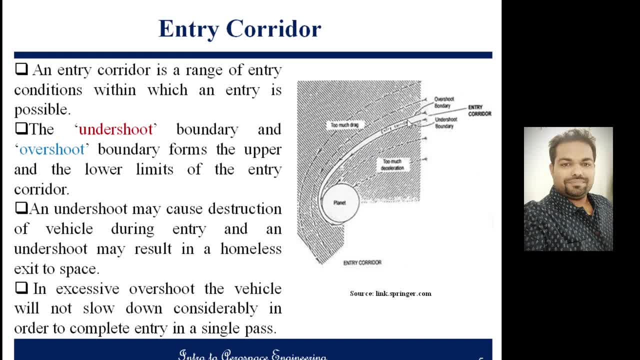 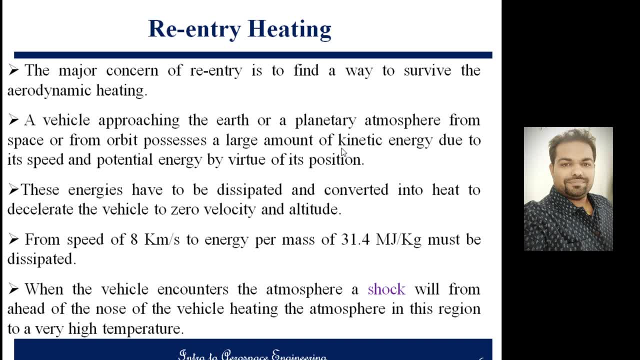 entry is possible and that is known as entry corridor. entry corridor. now, when we come, when we talk about the re-entry heating, this is the major concern of you know, space vehicle when they are entering into the earth atmosphere and how to survive. that is a big challenge. so a vehicle approaching 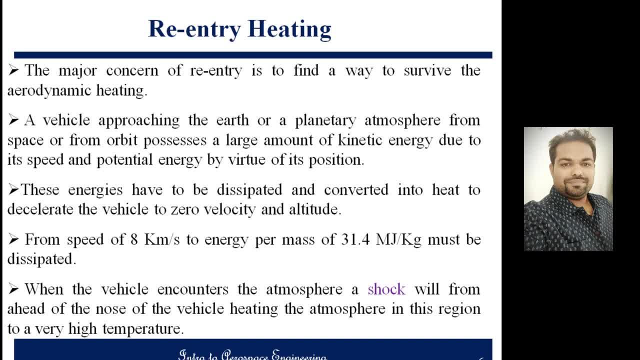 the earth or a planetary atmosphere from space or from orbit possess a large amount of kinetic energy due to its speed and potential energy by virtue of its position. so these energies have to be dissipated and converted into heat to decelerate the vehicle to zero velocity and altitude. 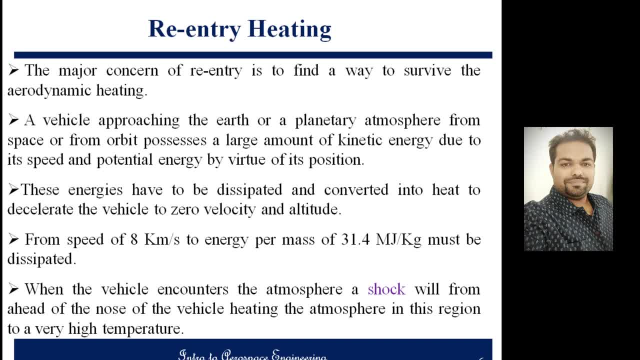 so from a speed of 8 kilometer per second to energy per mass of 31.4 mega joule per kilogram must be dissipated. so this much amount of heat need to be dissipated. dissipated then only you can slow down the vehicles. 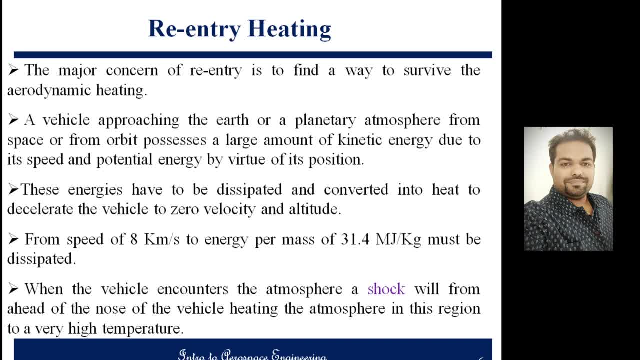 required for re-entry. so at high speed associated with re-entry from space, air cannot flow out of the way of the arm rushing spacecraft fast enough. so when the vehicle encounters the atmosphere, the shock, a shock wave, will form ahead of the nose of vehicle, heating the atmosphere in this zone to a very low temperature. 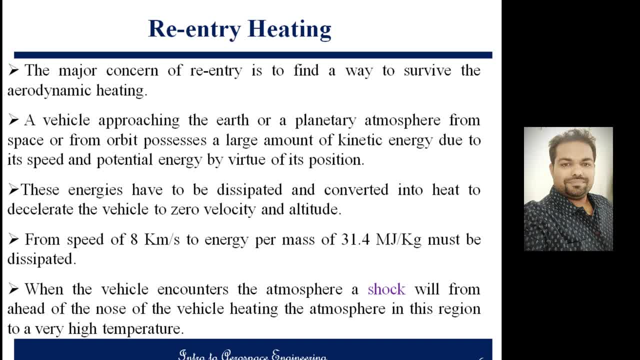 very high temperature. The moment it comes in contact with the Earth's atmosphere, a shock wave will form in front of the nose, will cause very, very high temperature rise. As the vehicle plunges into deeper and denser atmosphere, the vehicle will increasingly. 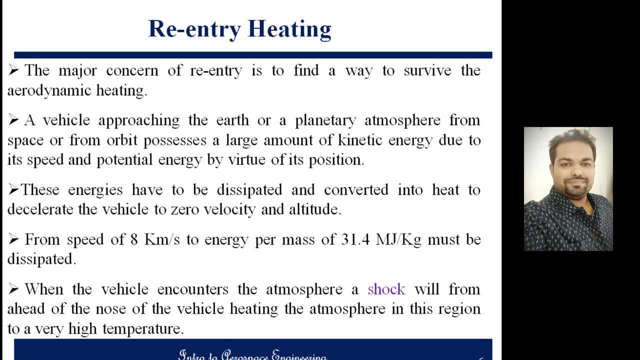 be heated by the atmosphere. Why? By developing the layer of incandescent atmosphere around it, while the speed of vehicle will continuously be reduced by breaking force of the atmosphere. In this manner, the vehicle's kinetic energy is converted into heat. If all the vehicle's 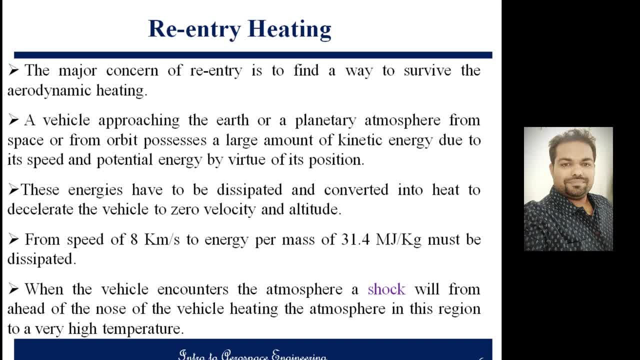 kinetic energy were converted into heat within the vehicle itself, it would be more than enough to vaporize the vehicle. That condition should not be existing. That's why I said that aerodynamic heating is a big, big challenge and we need to avoid it. We need to minimize. 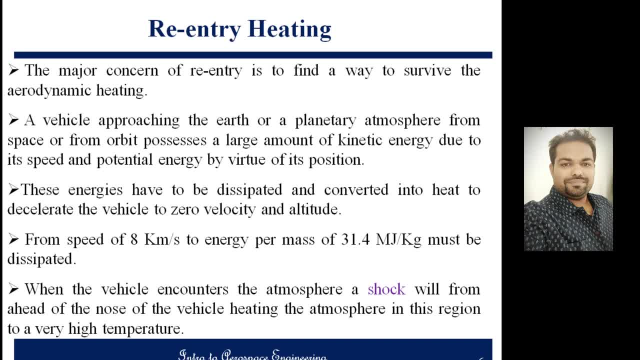 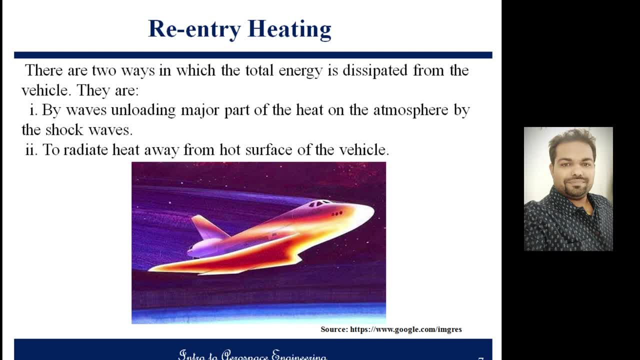 it, Otherwise it is very difficult to enter into the Earth's atmosphere. So there are basically two ways in which total energy is dissipated from the vehicle. First by waves unloading major part of the heat on the atmosphere by shock waves. So you design. 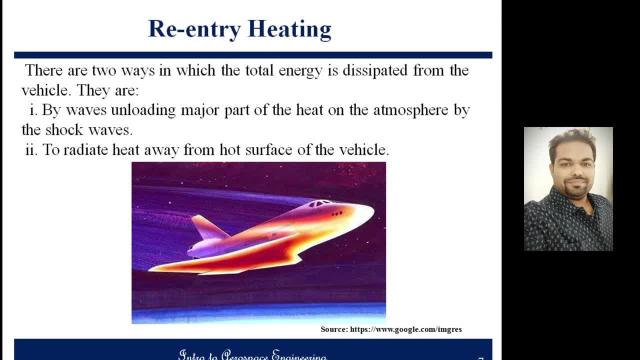 your front nose of the vehicle in such a way that shock should not attach over it. It should be detached so that you will have sufficient spacing between the shock and your vehicle. So it will be. it will not be direct heating of the surface, So a lot of heat will get dissipated. 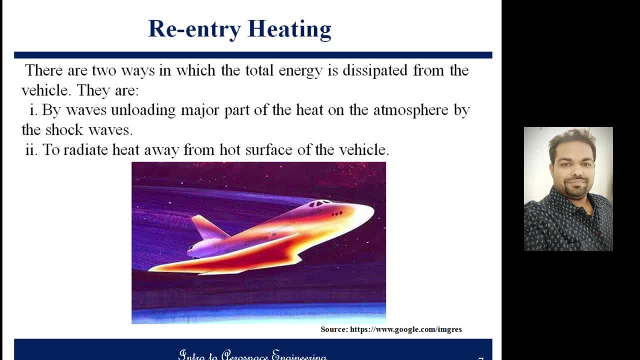 to the atmosphere. Second method is to radiate heat away from hot surface of the vehicle. So how, basically, this will happen? Look at this example: right, This is the space vehicle which is entering and this, this, this is condition of red hot. right, This atmosphere. 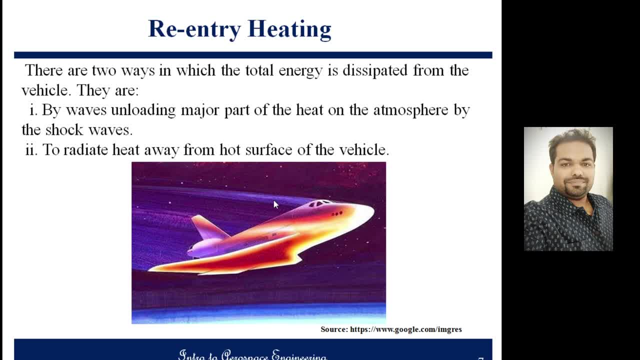 is complete material, It is becoming red hot. The movement is entering, The movement is entering into the Earth's atmosphere and this is the formation of shock waves. So usually for the spacecraft we make nose as a blunt nose right To avoid the formation of attached. 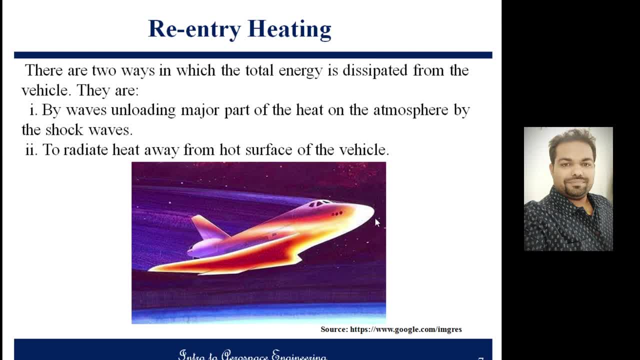 shock. But there is no attached shock, there will be no large aerodynamic heating. To avoid the large aerodynamic heating, there would be a- it is a bluff body, right, Bluff nose. In that case, shock will form a distance away from it. In that case, in that case, the surface, 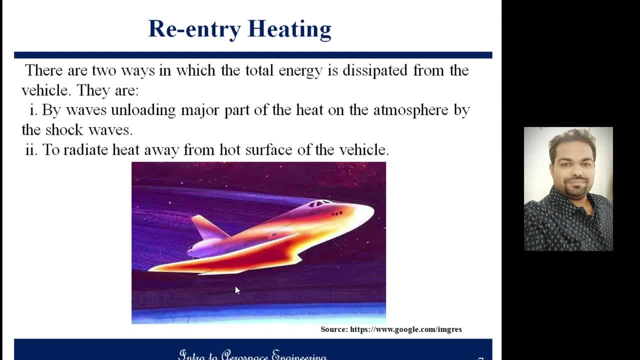 of the vehicle will be subjected to less heating. So diversion of heat by strong shock wave is the result of molecular interaction in the gas around the vehicle. When molecules strike the forward surface they bounce back, So many of the rebounding particles collide with the oncoming molecules, diverting them from the surface and preventing them by hitting. 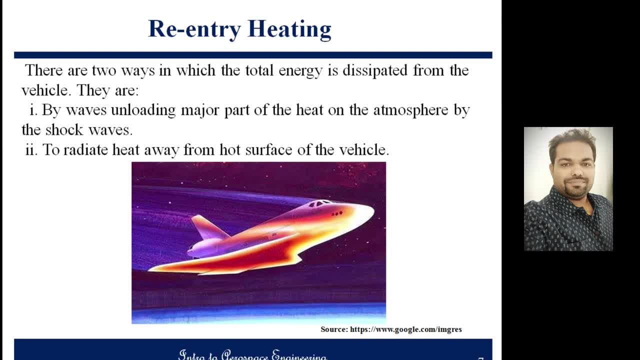 it by direct impact. A blunt nose produces the strong shock wave. Since the fraction of the total heat load that is transferred is directly proportional to the strength of the shock wave, the stronger the shock wave, the lesser will be the heating on the surface. That means when shock wave 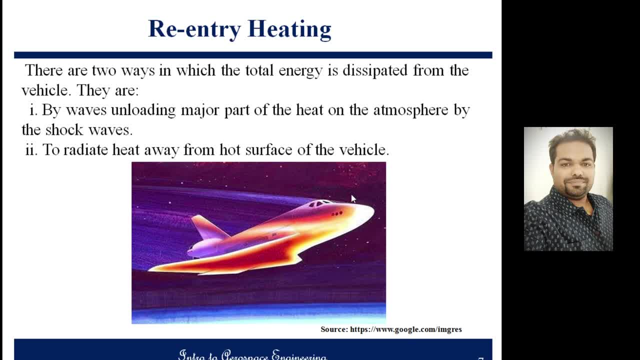 has formed here. so when flow coming molecules will strike over the surface and rebound back. When they are going back they will disturb the motion of the shock wave. So when the shock wave has formed they will not be directly hitting on the surface because of that Surface. 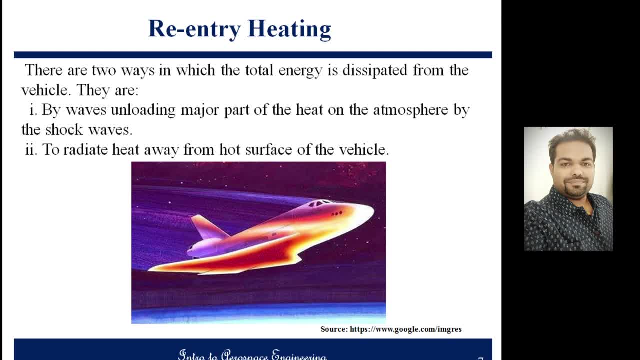 will be shaped from the direct heating. They will be dissipating back, So higher the strength of the shock wave, lower will be the aerodynamic heating of the surface, Higher the strength of the bow shock. we use that as a detached shock or bow shock. That is why. that is why. 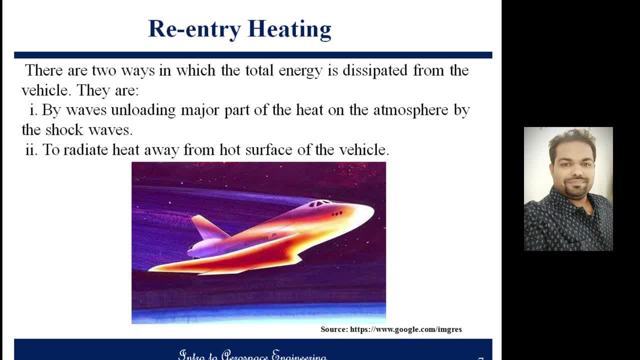 for a space vehicle. we make the front nose, We make the front nose as a blunt nose right. It is a blunt nose In that case. a shock, normal shock, strong detached shock will form right. Detached shock will be a combination. 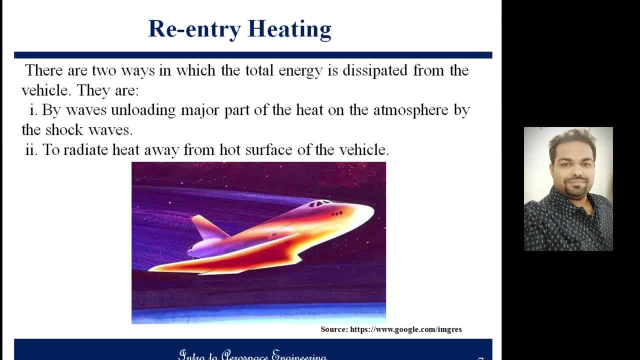 of means: a combination of one strong normal shock followed by two oblique shock. Oblique shock will have lesser strength compared to the normal shock, So immediately after the normal shock, flow will become subsonic. When flow is subsonic, there will be no aerodynamic. 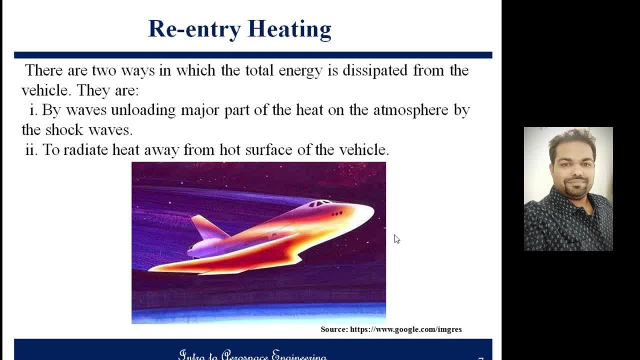 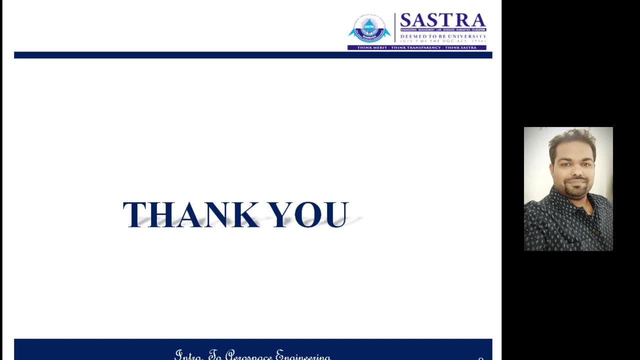 heating. That is why you know blunt nose is preferable And this aerodynamic heating is a big concern right particularly, we have to deal with, We have to deal with. So this is regarding the reentry vehicle right and aerodynamic heating. So with this I want 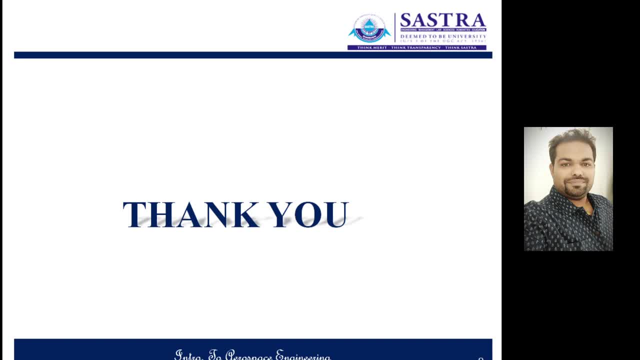 to close the today discussion right. If you are having any doubt in this, feel free to write in the comment section or you can directly ask to me. So, as a summary, today you have introduced about the reentry vehicle: what are the reentry vehicles and what are the? 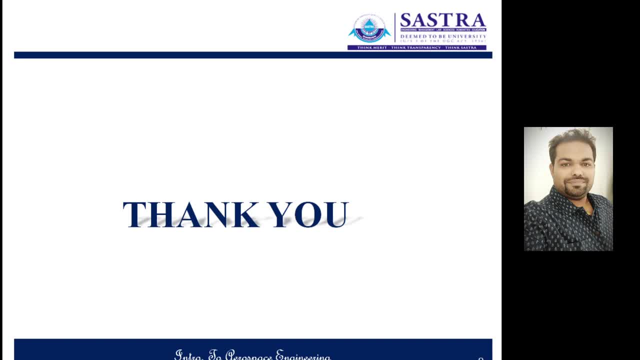 big challenges of reentry. You have been given a clear idea about entry corridor. There is a particular passage through which only reentry is possible. right, Successful reentry is possible. Otherwise, if you are going either downside or upside of it, right upper boundaries. 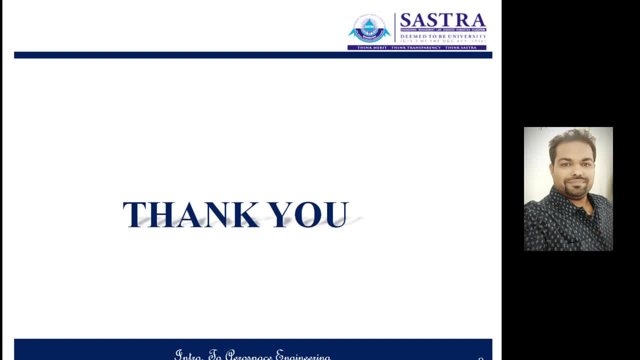 or you know, lower boundaries of it vehicle will face a lot of difficulties. So this will be a lot of problems and reentry will become difficult or almost impossible. And finally, you have given a clear idea about aerodynamic reentry heating- how it is going. 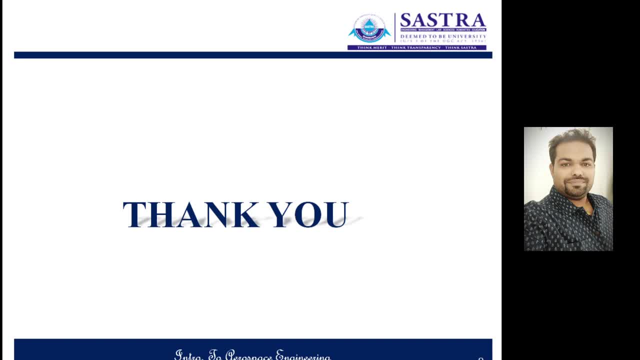 to impact over the spacecraft And also you have been given a clear idea about how to minimize it. We cannot avoid the aerodynamic heating, but you can minimize. There are various methods of the spacecraft. we are using the thermal protection system that is called thermal. 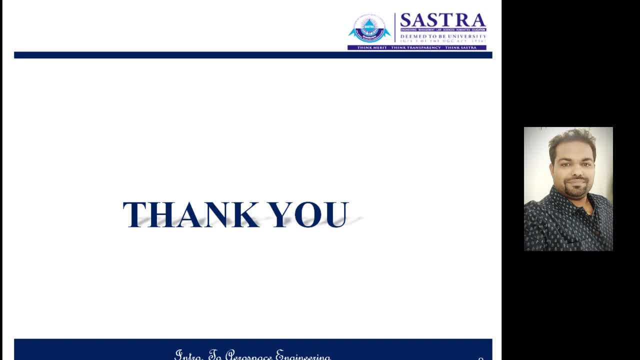 shield. so front nose will be made by the special material so that will be attached as a thermal shield at the nose. or some space vehicles we are using even a thermal barrier coating to avoid the air when I am heating and most of the space vehicle front nose, if you look at, or spacecraft. 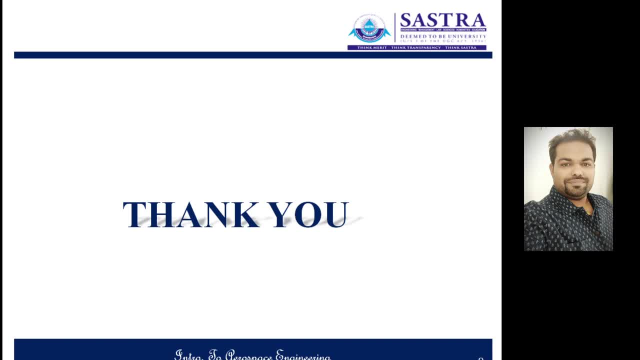 front nose, if you look at that, will be blunt nose. it is having more like a circular cylinder. so, due to which, what will happen? when it interacts? right the earth, atmosphere at hypersonic speed, right there will be formation of shock wave and shock wave will be a detached shock wave and we 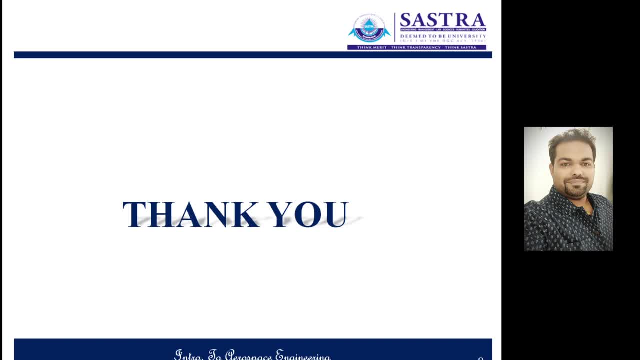 prefer to have detached shock wave in order to minimize the aerodynamic heating. so if it is a trace of a air flow will not have direct interaction over the boundaries right? or you can say within the boundary layer. so within the boundary layer heating will be less compared to the outside of the boundary layer. so outside of outside.